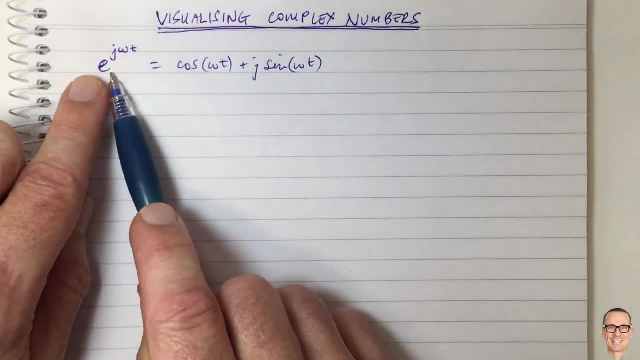 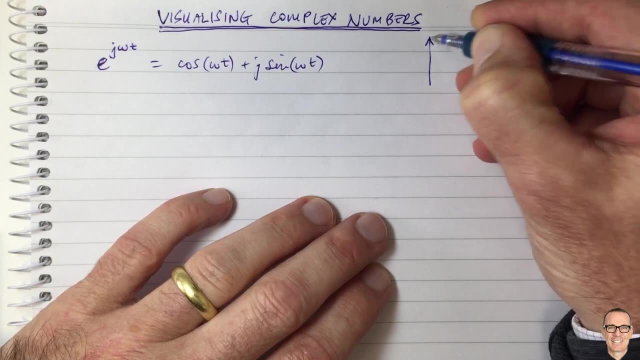 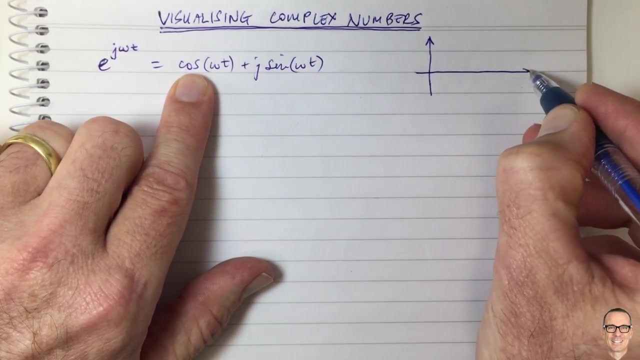 about these waveforms, And the first thing I do is, when I see a complex number, I think about a waveform and I think about the cos wave form. So here's, because that's the real part. but also, of course, sine waveform is also of the same shape, just with a different phase offset. So I'm going to 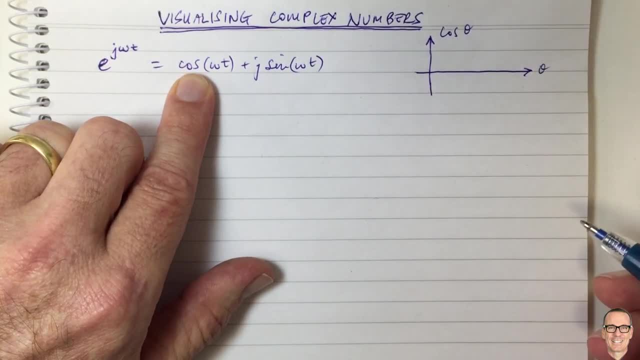 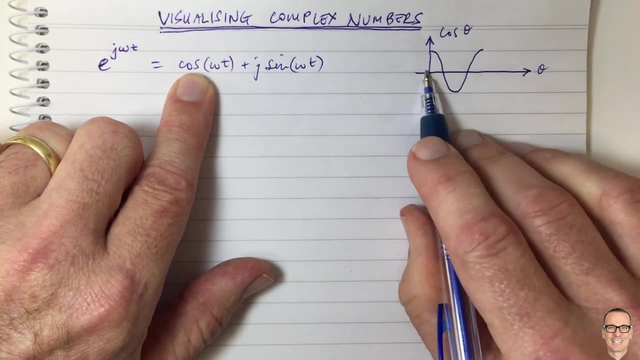 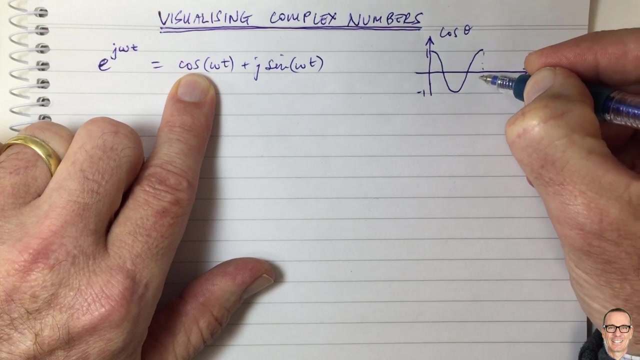 draw here cos of theta and I'm going to plot it with respect to theta. and that cos waveform starts, or the cos function starts when theta equals zero, starts at one and then goes- looks like this- goes to minus one and goes through an entire cycle in two pi, So in two pi in radians. Okay, so this: 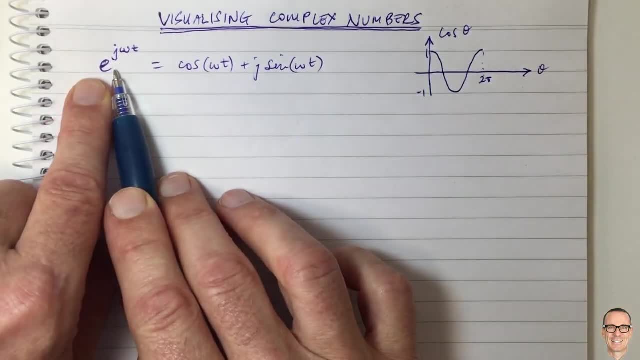 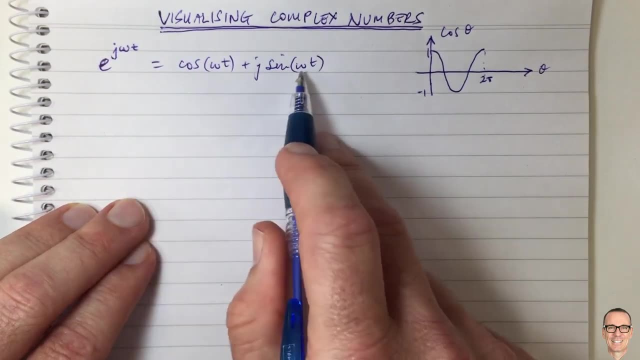 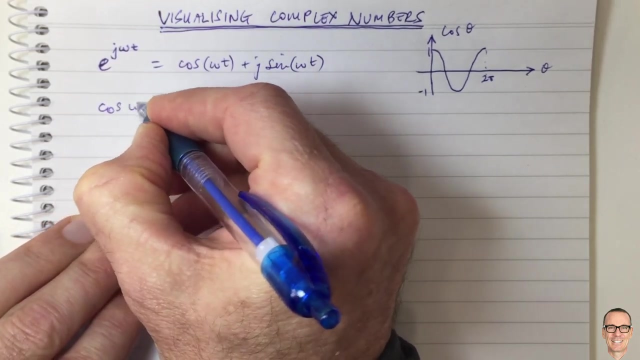 function here I think about when I see a complex number, and I encourage everyone to do that, Okay, so what's another thing that we, another expression of this, in fact almost the reverse way, where we can represent cos in terms of complex numbers, So cos of omega t- again another standard. 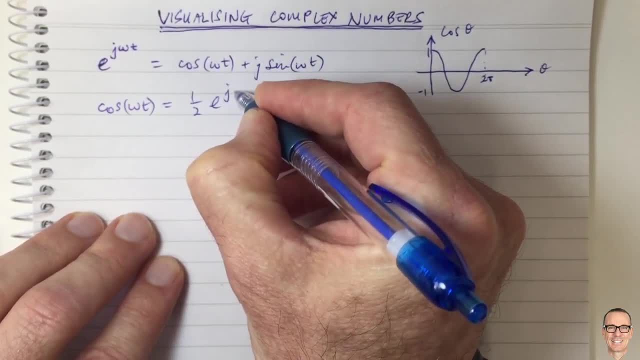 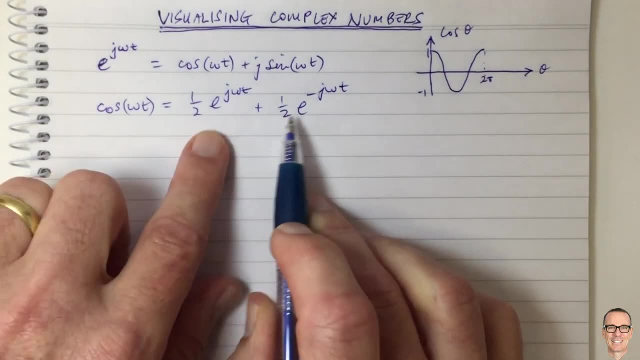 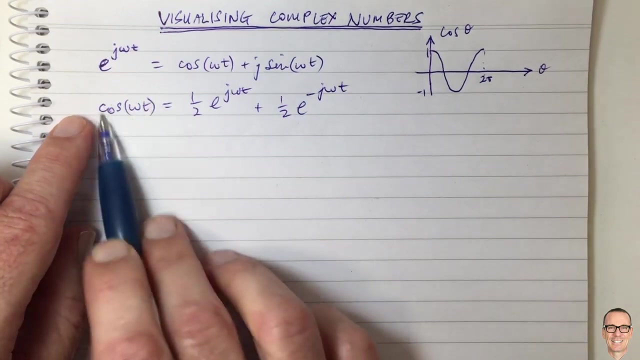 expression, standard way of representing it is e to the j omega t times a half, plus again a half times e to the minus j omega t. And so this way here is going from complex numbers in polar into Cartesian, and this way we're going here from a real function which we think of. 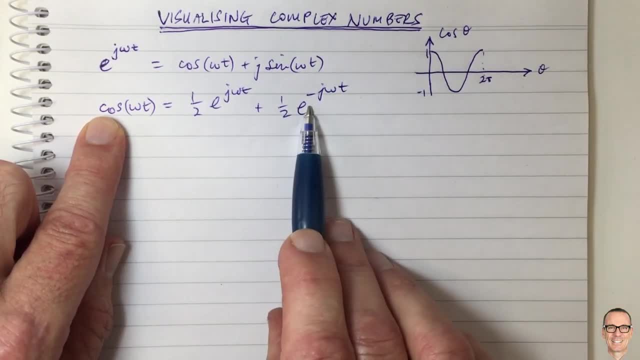 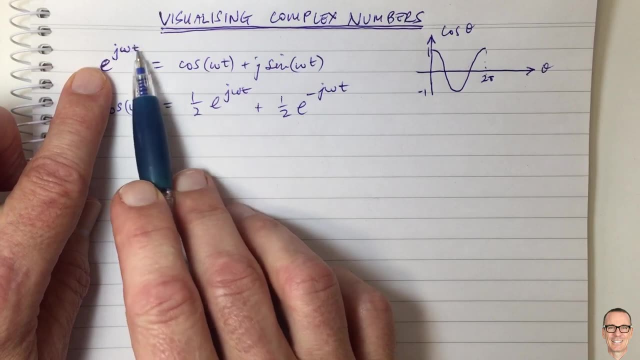 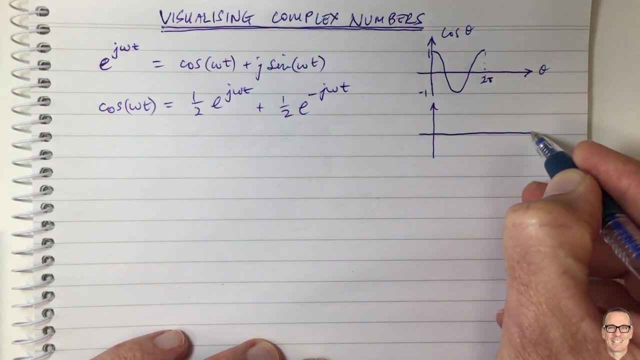 in terms of this cos shape, and we can write it in terms of complex numbers. Okay, now let's think a little bit more about this complex number, This one here. I've got a time coefficient in there, and that's why I always like to think of it in terms of a function in time, a sine wave or a cos wave changing. 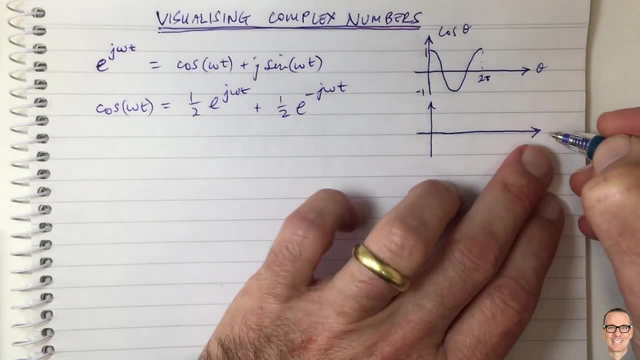 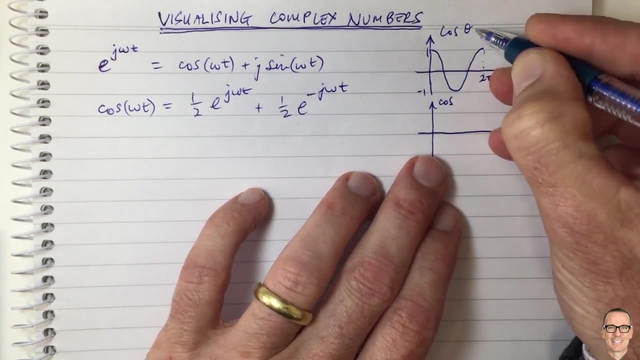 in time. So let me actually draw this in terms of something we're more familiar with, with frequency and time. So let me plot here cos we've got, cos of theta. here we've plotted with respect to theta. let's do cos of 2 pi f times t. So 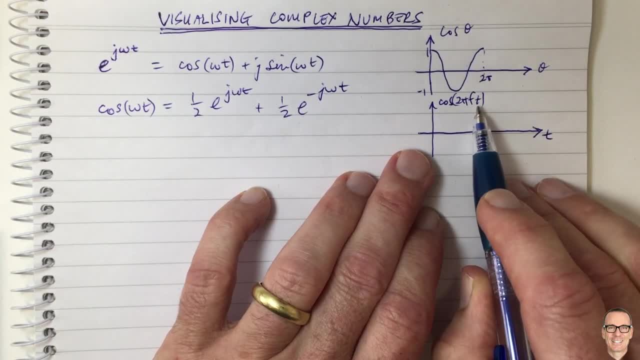 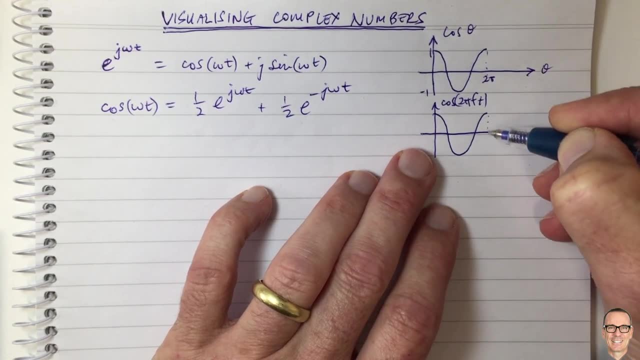 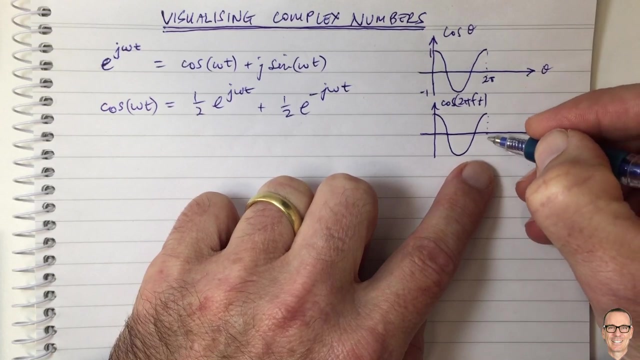 this is a cos wave form and a certain frequency f and of course it changes with time and it of course has the same shape as this waveform above. but now we're plotting with respect to t, which is only part of what's in the brackets. So now I think you can see here that what's. 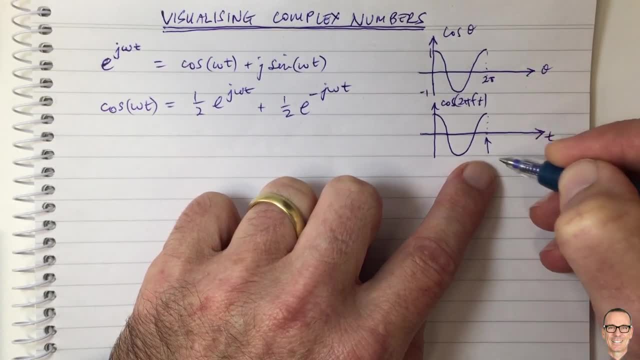 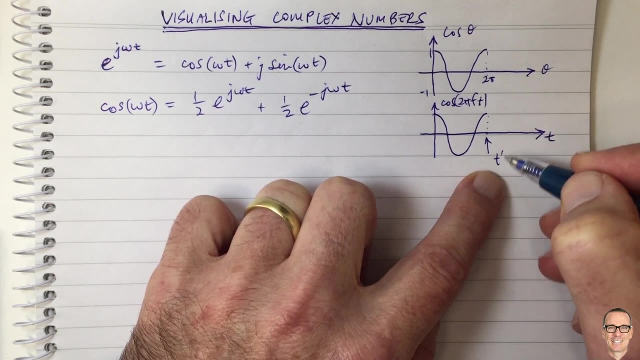 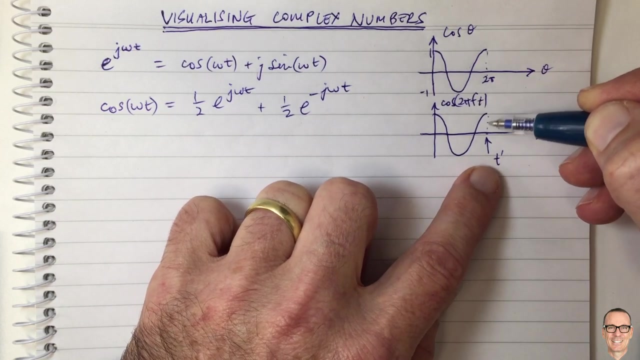 in terms of plotting with respect to t. what value is that time there? Well, that's the period of the cos waveforms. I'm going to call that t prime. and that happens. that t prime happens when, when f equals 1, because when f times t, 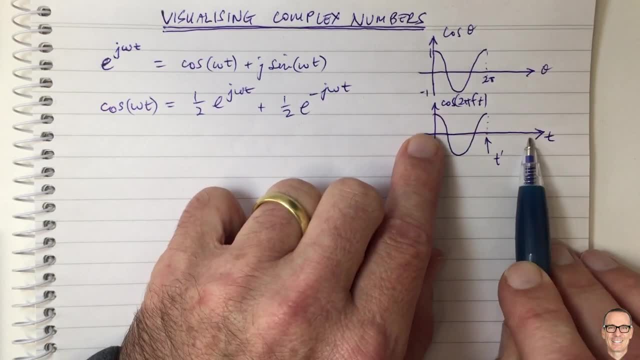 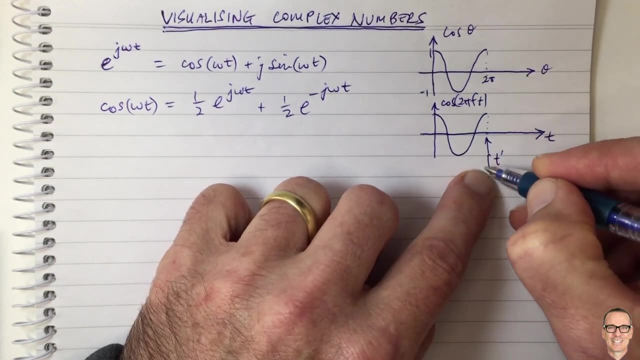 equals 1, you'll have cos of 2 pi in the brackets here and that's the same up here when you have cos of theta, when theta equals 2 pi. So when f times t prime- because t prime is the period when that equals 1, you have completed an. 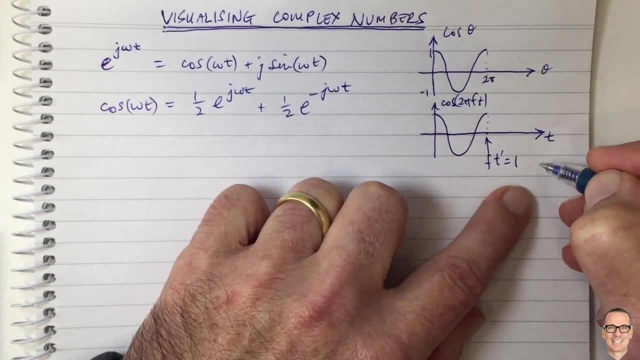 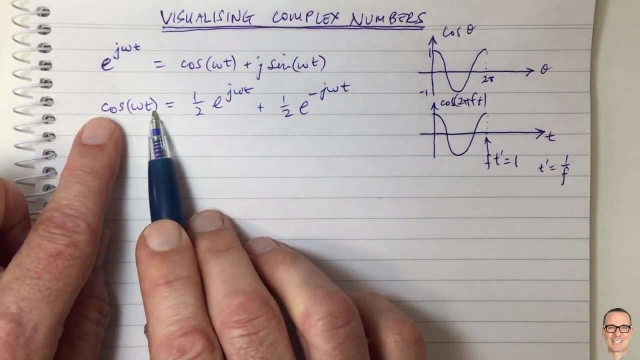 entire period of this cos waveform, And so the period therefore equals 1 divided by f. Okay, so this is a cos waveform and that's what we're plotting over here, that's what we've written out over here and we've written it into. 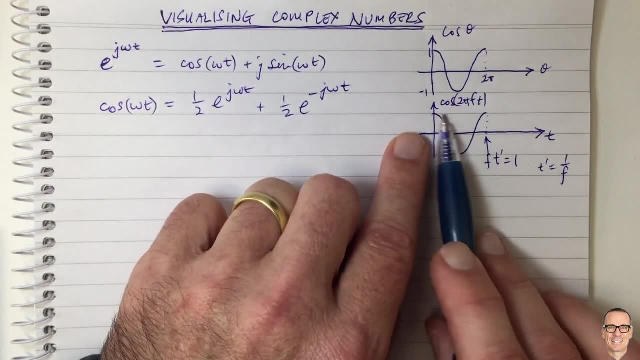 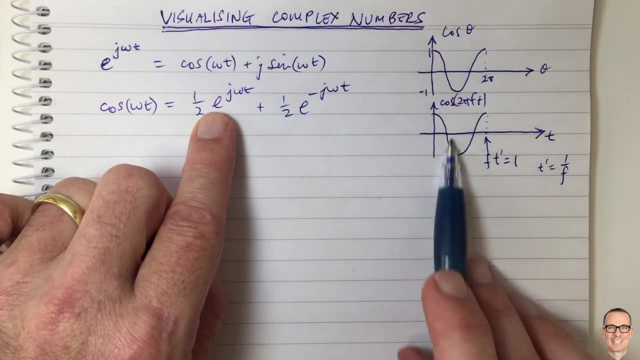 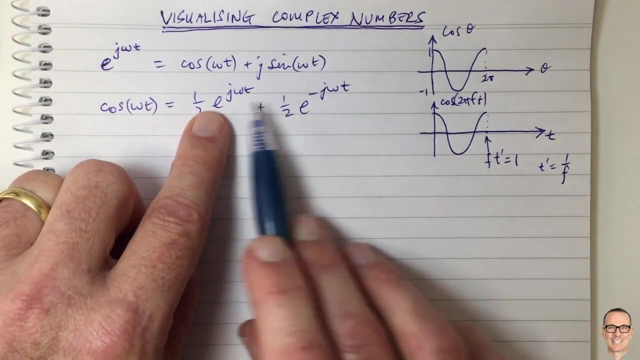 terms of two complex numbers. But again, I'm thinking of this waveform and when I'm looking on the left and then when I'm looking on the right, I'm also thinking: well, these two numbers here equal this waveform. These are both complex numbers. this waveform is real. so in this case, the imaginary parts of 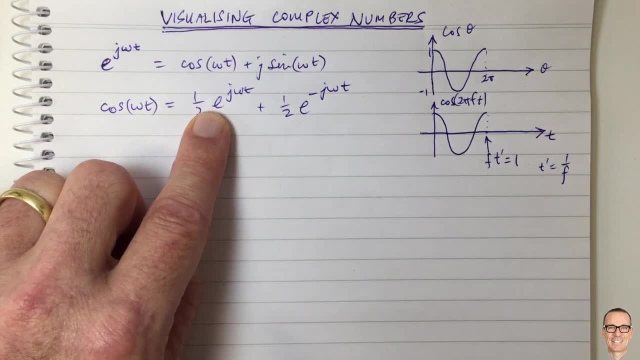 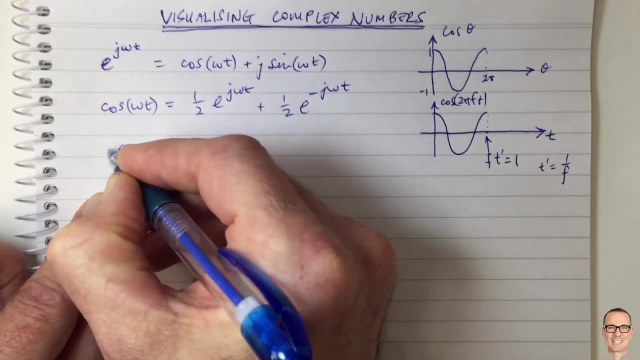 these two complex numbers cancel each other out, and that's an important concept to know about. Another thing is when we have a complex number that doesn't have time involved, So let me write another one here and that's the time that's in here. So I'm going to write down e to the j phi. So this is a complex number here. 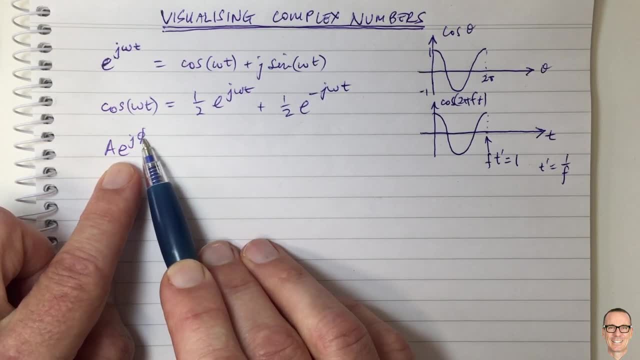 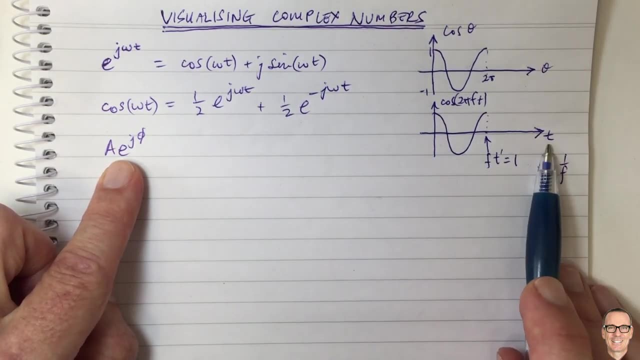 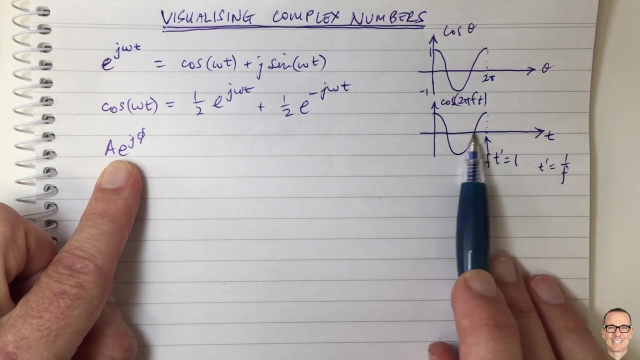 it has an amplitude of a and it has this term phi in here in place of omega t. So now, when I see this, I'm not thinking of a waveform like this anymore. that changes with time. I'm thinking now instead of a phase, and I'm thinking of a phase change to this. 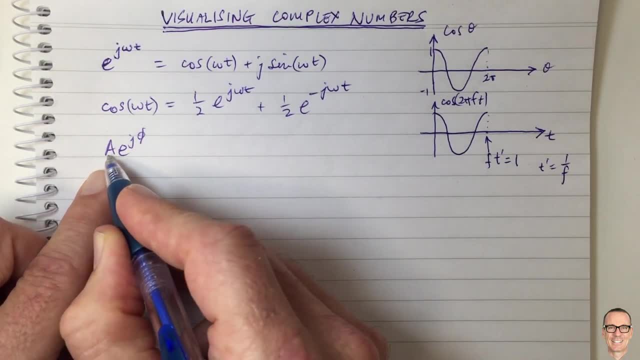 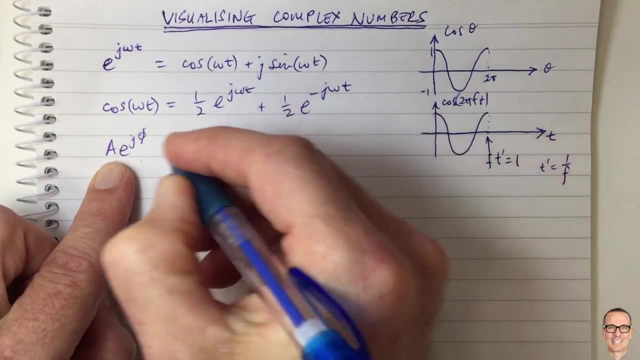 kind of a waveform. So why do I think about that? Well, let's think that if we had this number and let's say we multiplied it by this complex number above, So let's say e to the j, omega, t. Now, just to remind you, when I see this complex number, I'm 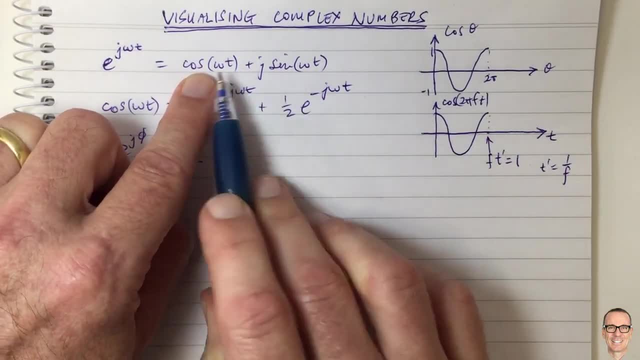 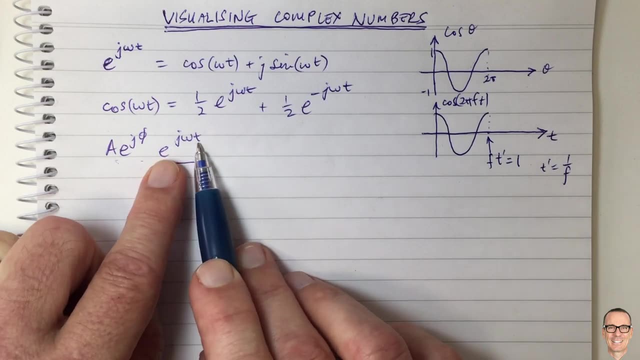 thinking of a cos waveform in the real part and a sine waveform in the imaginary part. So this is what I think of when I see this. So I see this and I've got a t in there, and I'm thinking about waveforms that look like this. So what happens when we multiply? 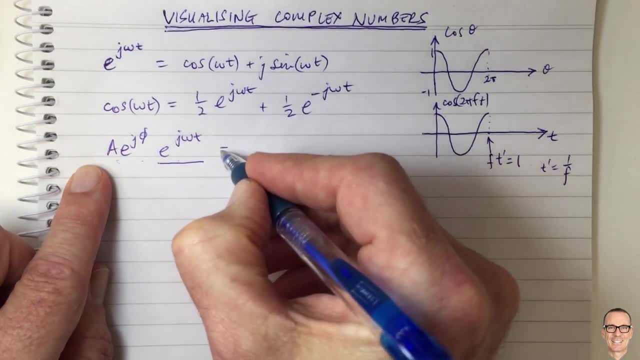 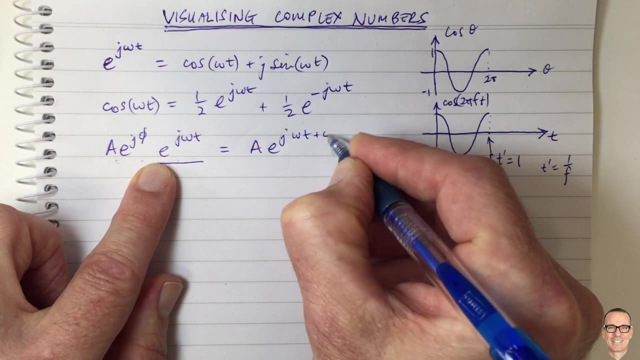 this by this one here. Well, of course we can collect the terms in the exponential. So this gives us a times e to the j, omega, t plus phi. Okay, so now we've got a new complex number and it does have the t in there. So once again, I'm thinking. 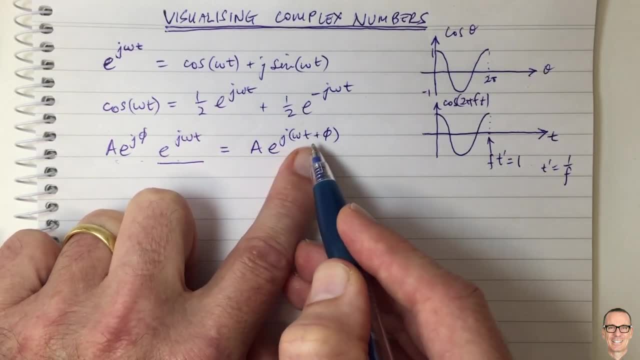 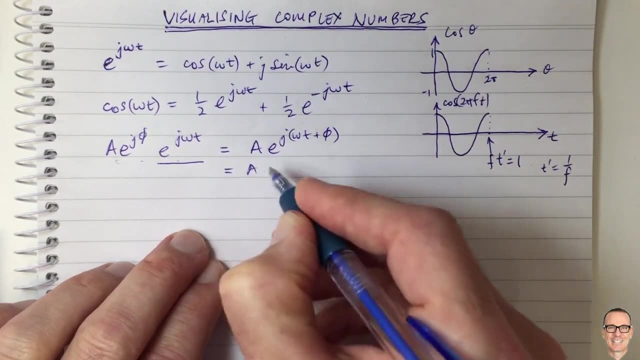 about these waveforms here, but it's obviously now a waveform of a cos form with a phase offset, And I'm just going to use that first formula up here just to remind ourselves. this equals a cos of omega t plus phi plus j sine phi. 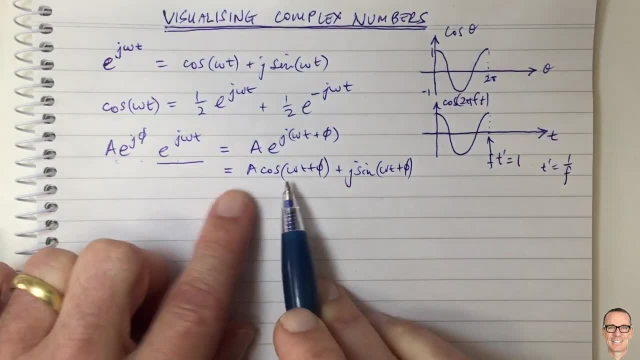 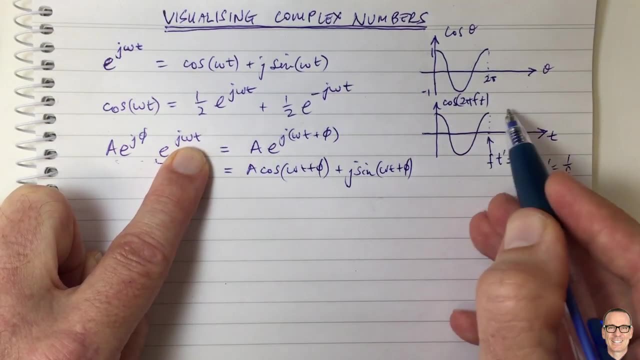 So we know that the time cross is the sum of omega t plus phi. Okay, so when we take a complex number, which is, which has a time coefficient, which means it's a time varying function like this, a cos function and an imaginary sign if we multiply it by something. 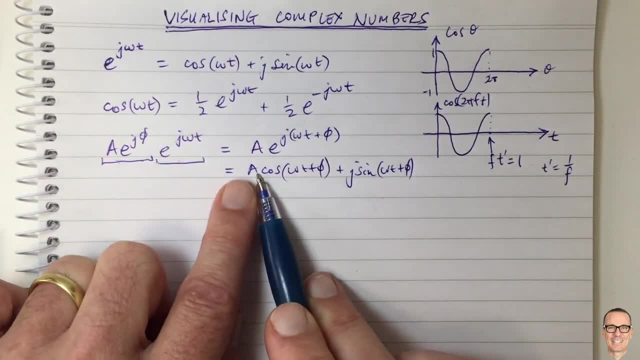 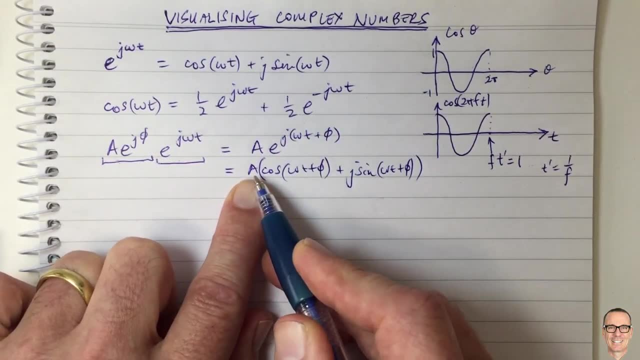 which doesn't have the time involved, then what we're doing is we're multiplying it by an amplitude- and, sorry, we should have an a in here as well. I've put brackets around that. We're multiplying it by an amplitude, We're scaling it by an amplitude. 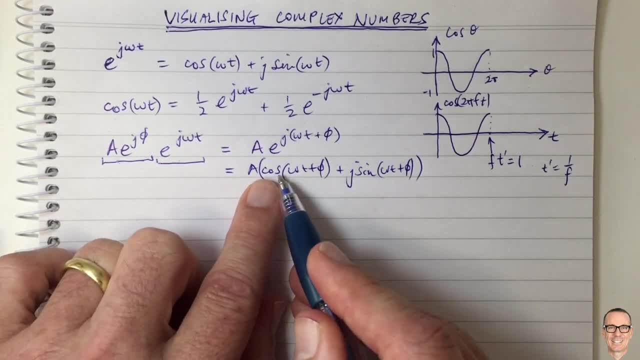 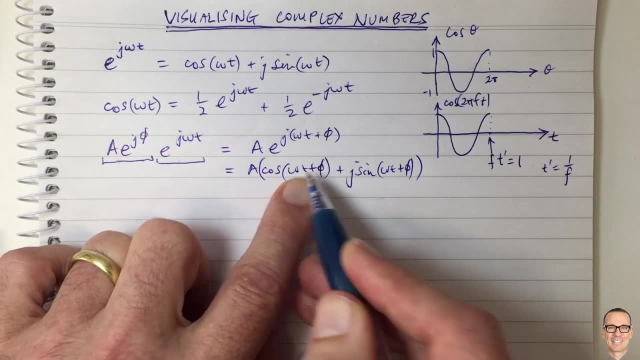 and we're also changing the phase. So we've got cos instead of just cos omega t. we've now got cos omega t plus that phase offset. So what that means is, when time equals zero, this function is not this cos anymore. 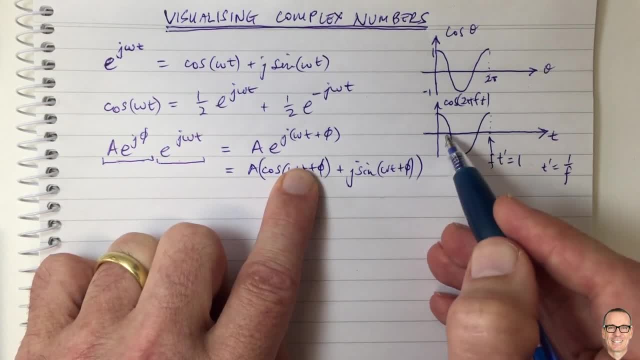 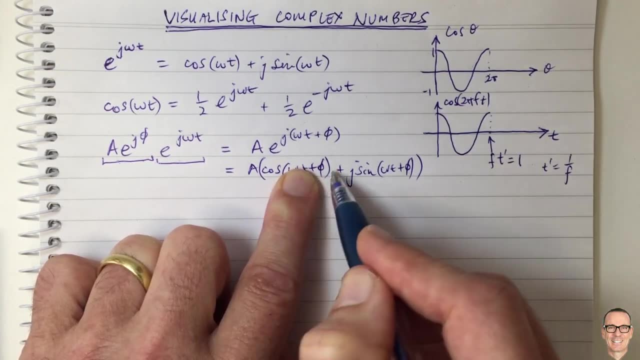 it's the shifted cos. So when time equals zero, we're going to have the value of this cos waveform here when the cos of phi. We can find out that cos of phi by looking up here, because this is just as that as a parameter. 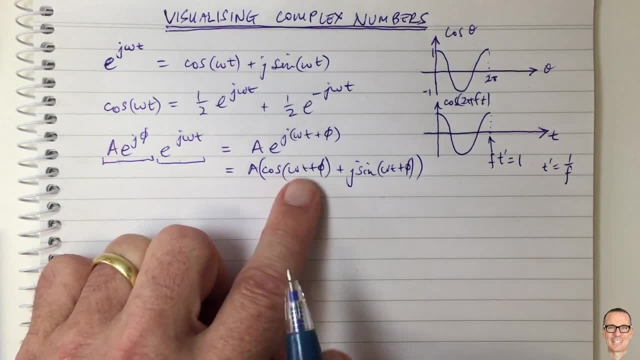 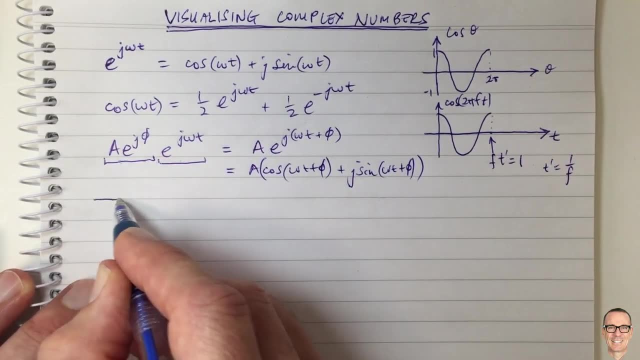 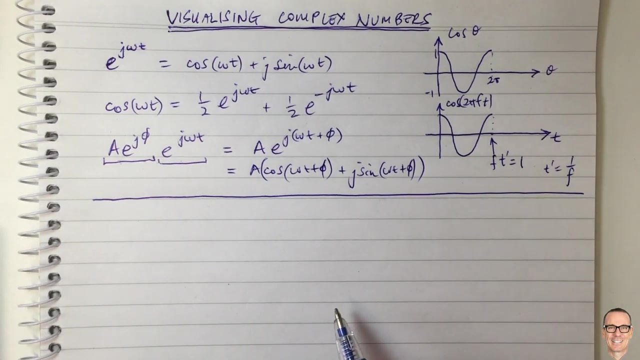 So it's a time-shifted version of the cos waveform. Okay, so these are all the basic things about, I think, visualising in imaginary numbers in terms of sine waves and cos waves and their various relationships. Let's look at an example. 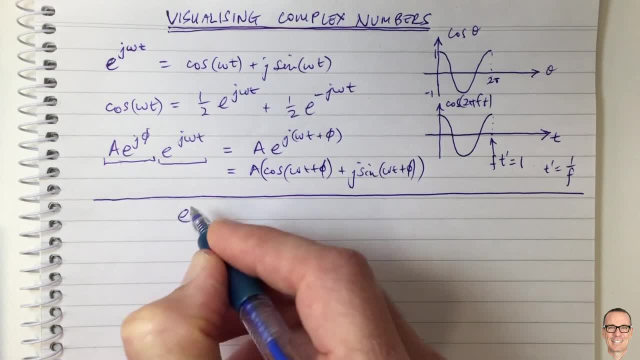 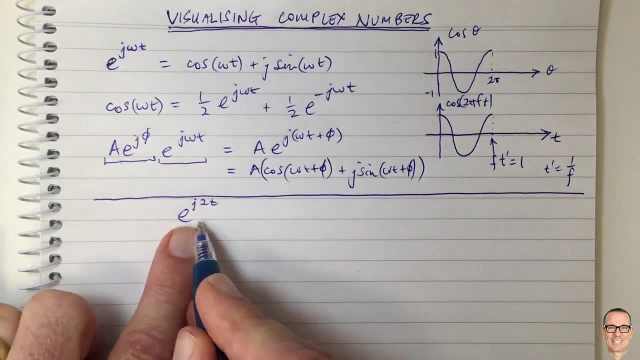 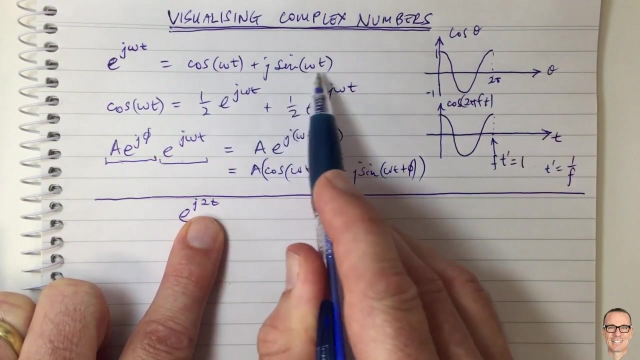 So let's say we had an example where we've got an equation or a complex number here, E, So that's immediately. we see the time in there. so we should be thinking about a cos waveform in the time domain for the real part. 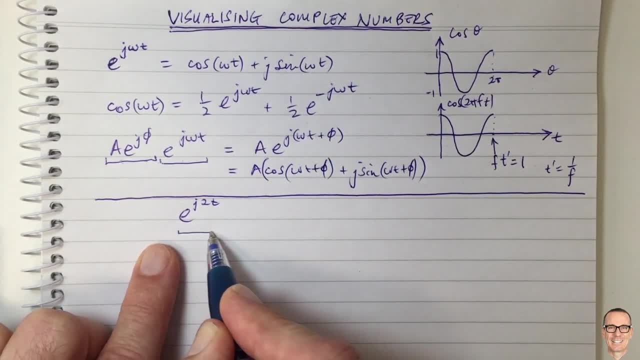 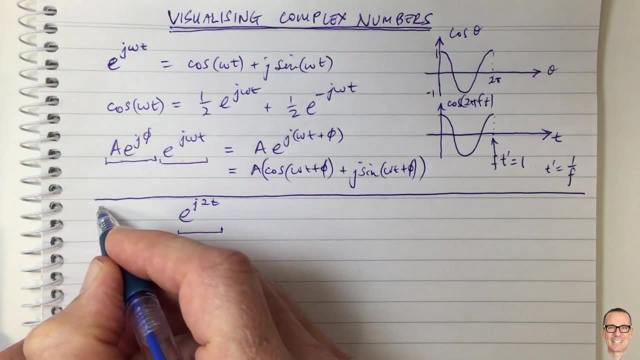 and a sine waveform for the imaginary. So when I see this complex number again, I'm thinking about waveforms, because there's a time in there. I encourage you to do the same. And let's say: this was being multiplied by minus 3, divided by 2. 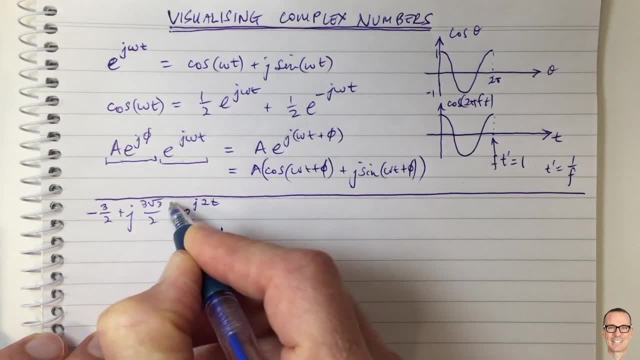 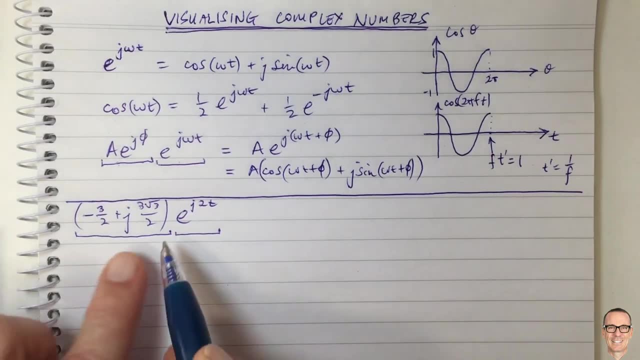 plus j3, square root 3, divided by 2, just as an example. So let's look at this example here. It's two complex numbers multiplied together. One is in the polar form, That's this one here. The other one is in Cartesian form. 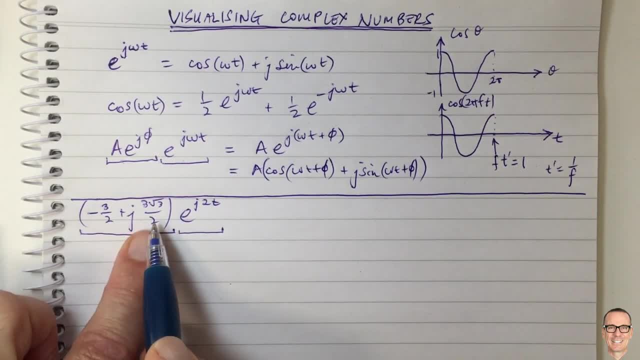 That's this one here. Now, this is a complex number that does not have time involved, So I'm thinking of it in the same way as this one up here. So I'm expecting, and what will happen is this number here. the effect of it will be. 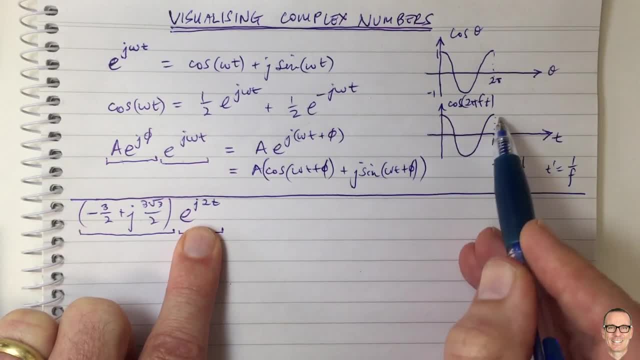 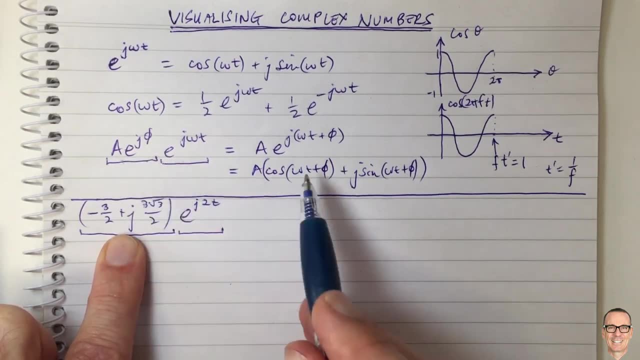 to multiply this wave, which is a waveform because it's got time involved. it's going to multiply this by an amplitude and give it a phase shift, Exactly like we saw up here. So we're going to have causes here with an amplitude and a phase shift. 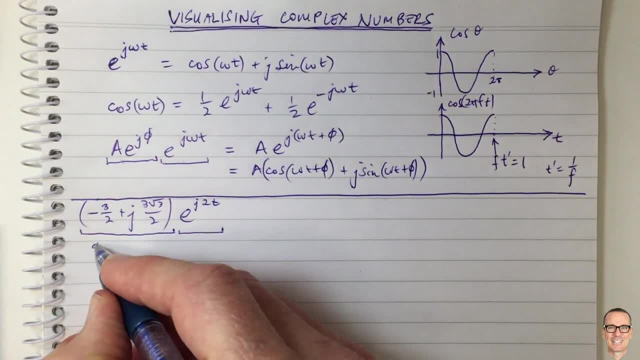 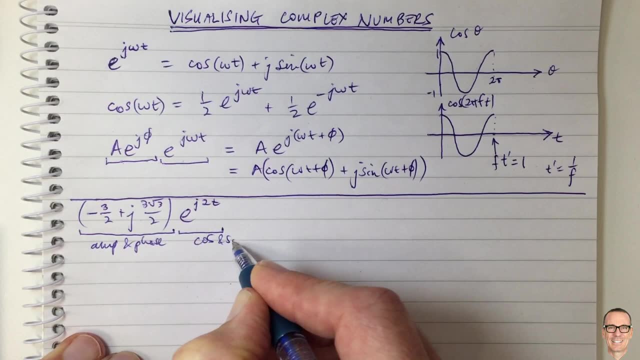 So let's use this example to work this out. So, as I say, this has got an amplitude and a phase. That's the effect of this one, And this one is cos and sine waveforms. Okay, and that's the important thing. 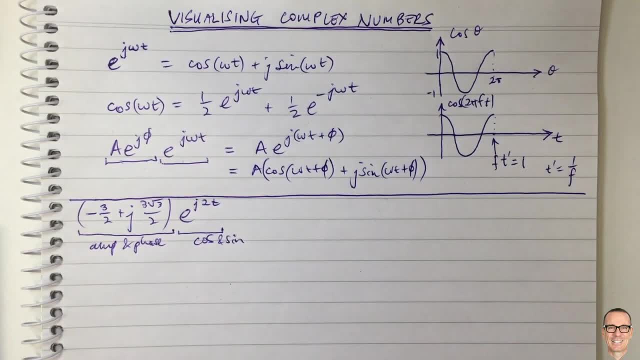 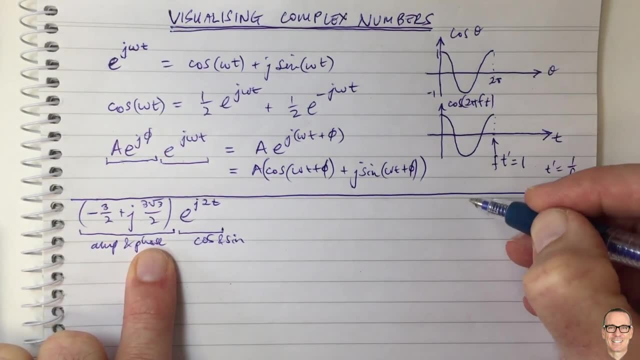 That's got the time function in it, Okay. so let's think about this multiplier out the front And let's first of all actually let's plot this Again. we're talking about visualizing it, So I encourage you to. 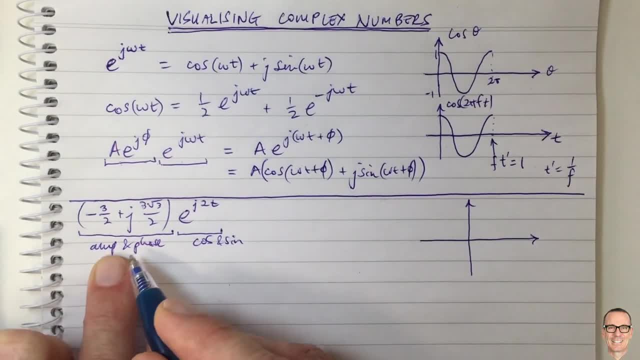 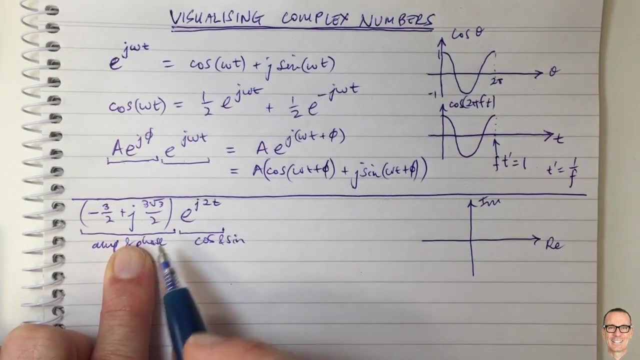 always visualize the complex number. So let's visualize this complex number. It doesn't have a time aspect, the one in the brackets, in terms of the real and imaginary. Let's at least plot and think where it is Okay. so the real component is minus three on two. 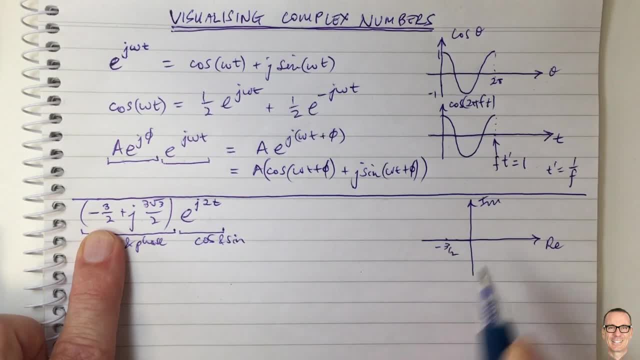 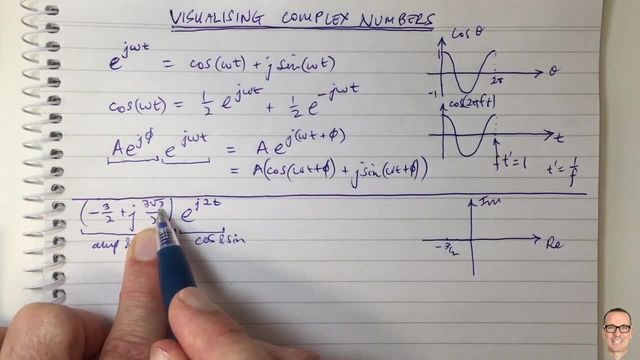 So that's this direction here, by minus three on two, And then it's got plus in the imaginary direction of three on two times square root of three, And square root of three is bigger than one, So that's going to be a bigger vertical height. 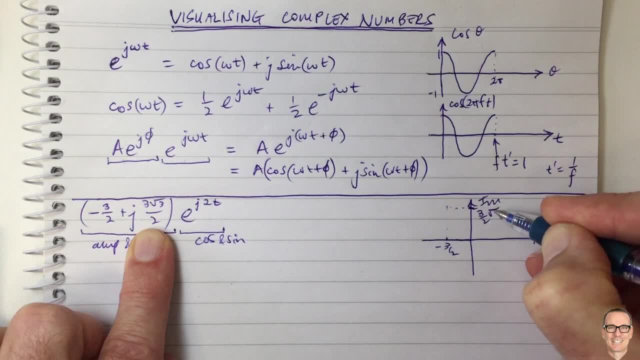 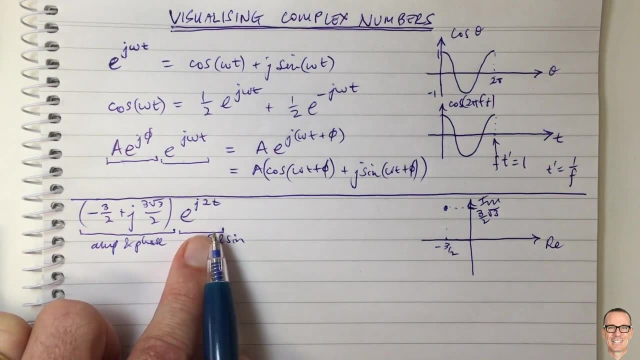 Up here and we're going to have that. That's three on two times the square root of three. So this is our complex number. that's out the front of our cos and sine wave in the way we're visualizing things. Okay, so what is this? 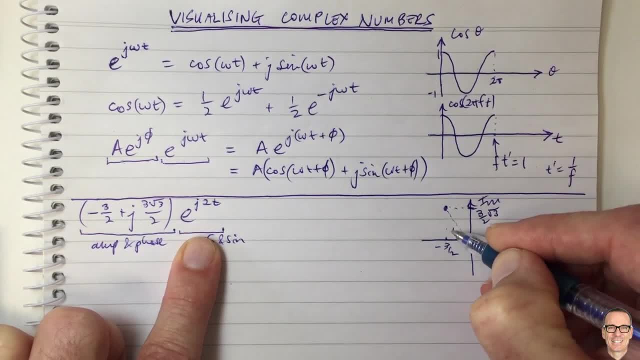 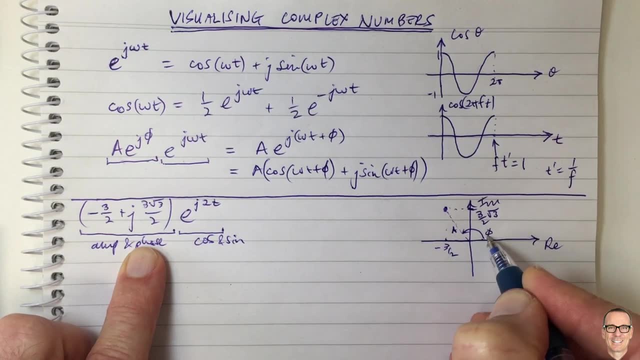 Well, that's something that has an amplitude of that distance there. So that's the amplitude A, And it has a phase. We always measure the phase from the real axis, So it has a phase here, phi around like this, So it's got an amplitude of the distance out to there. 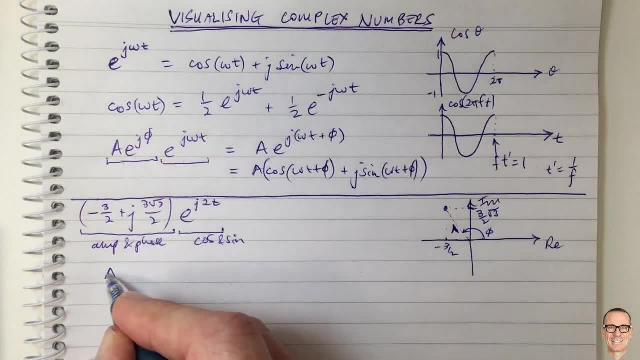 And that phase. So let's work those things out in this example. So the amplitude equals. well, of course it's the Pythagoras, So it's the square of the reals plus the square of the imaginaries, all square rooted. 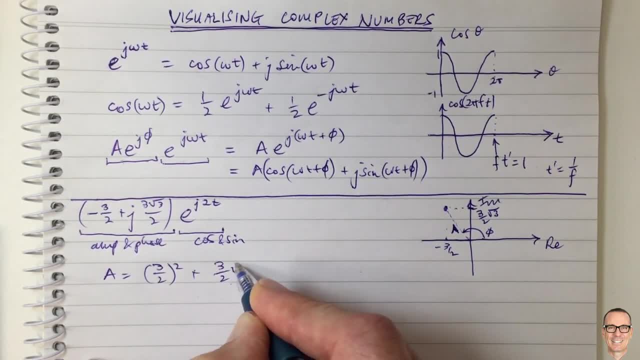 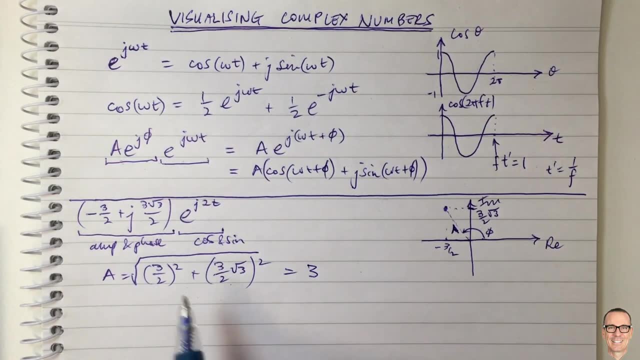 So that's three on two squared plus three on two times square root of three squared, all square rooted, And that equals three. in this example, That equals three. Okay, so the scaling is going to multiply our cos and sines by three. 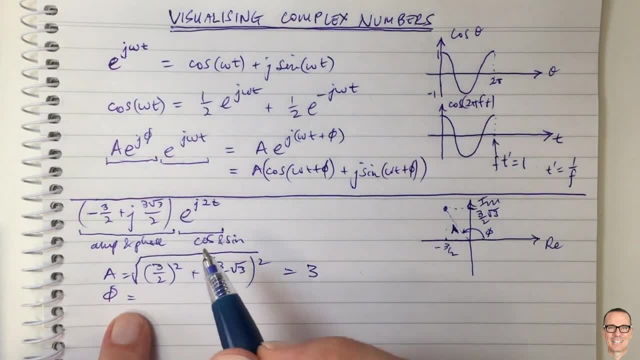 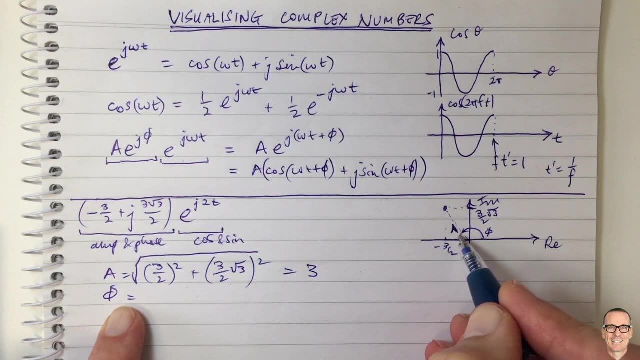 Okay, what about the phase? Well, the phase, we can see that here. Well, this is a phase that's bigger than 90 degrees. So we can work out the phase in here that's less than 90, and then do 180 minus that. 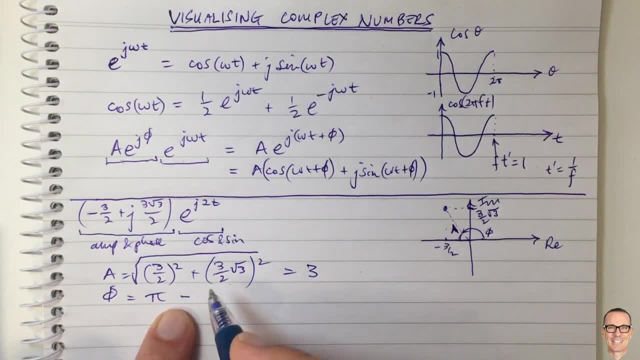 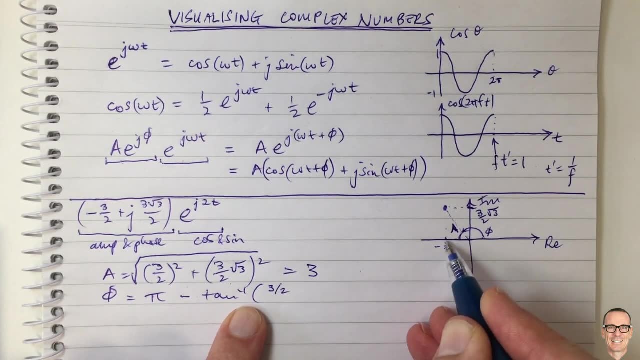 So it's pi and we're working radians. So pi minus the inverse tan function of the opposite over the adjacent. So it's the three on two because that's that distance there. Sorry, three on two, square root three, because that's the opposite divided by the adjacent. 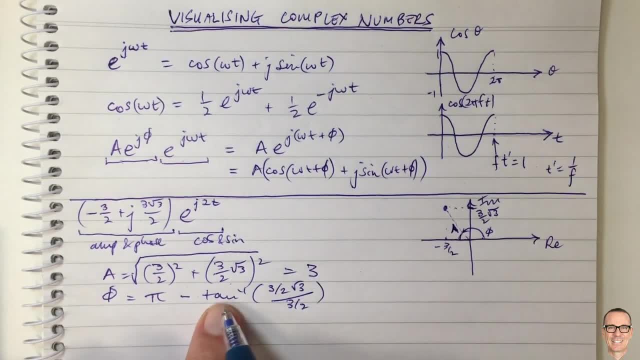 Okay, So that's the adjacent, which is three on two. So you've got inverse tan of square root of three, because the three on twos cancel And this equals, and you've got pi minus that, So this equals. I'll write it out: pi minus pi on three. 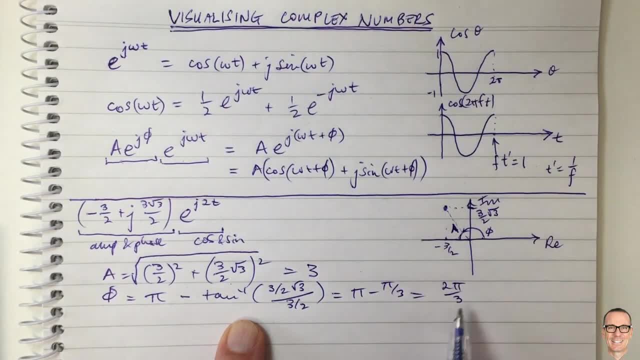 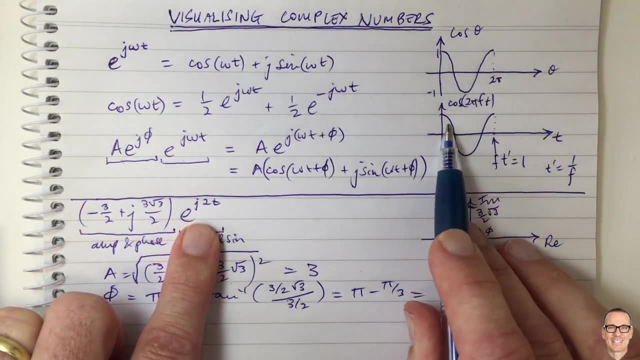 which equals two pi on three. Okay, so what we're doing here is this complex number, these two complex numbers multiplied together. We're visualizing this as a cos waveform. We're visualizing this as an amplitude and phase. It's amplitude scalar. 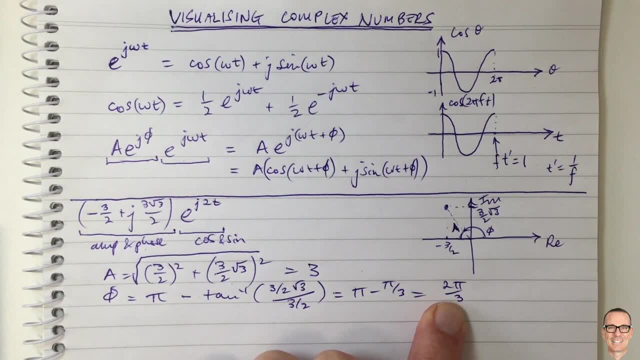 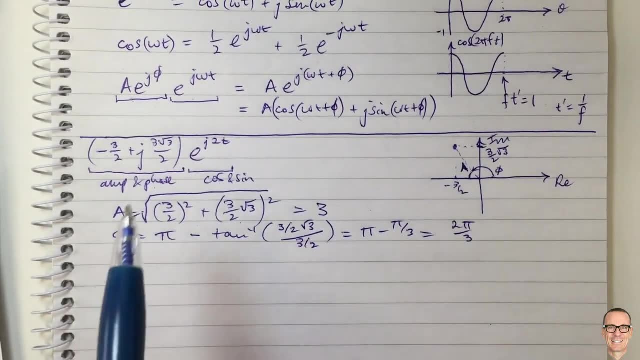 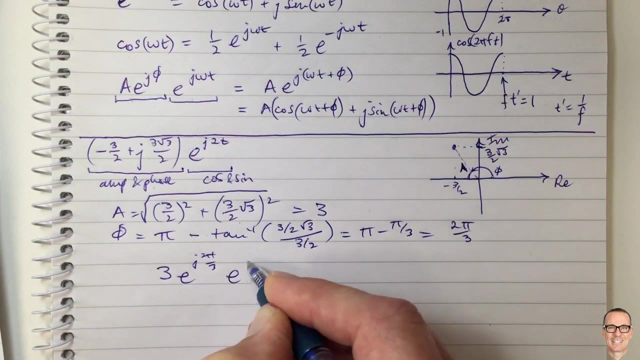 Scalar by three and a phase rotation of two pi on three. So the overall resultant complex number is obviously the multiplying these two together. you're going to get three times e to the j, two pi on three times e to the j two t. 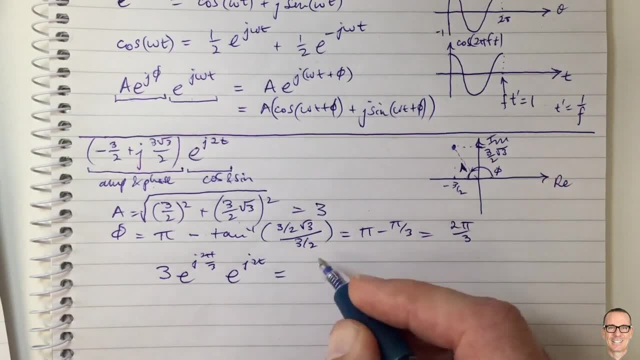 That's just simply writing this exactly out, And that therefore equals- I'm just going to write it in, or maybe I'll write it in: the real and imaginary: equals: three Cos two t plus two pi on three. This is going to help us to visualize it. 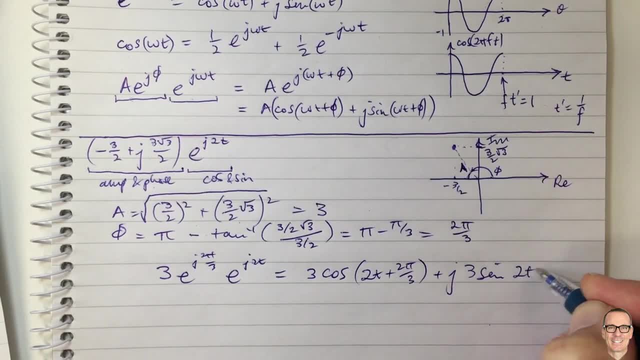 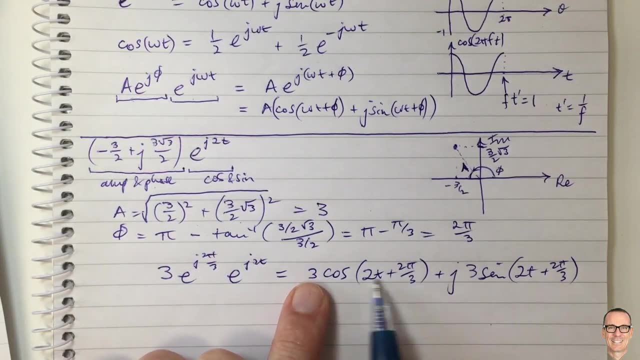 Plus j, three sine two, t plus two pi on three. And so maybe the last thing to do in terms of visualizing is let's maybe plot the real part of this and just link these complex numbers to real waveforms like the ones we had up here. 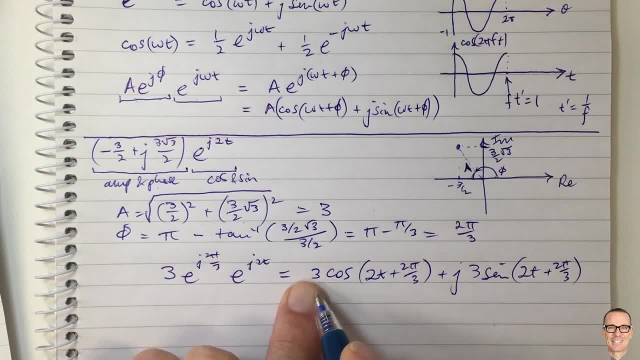 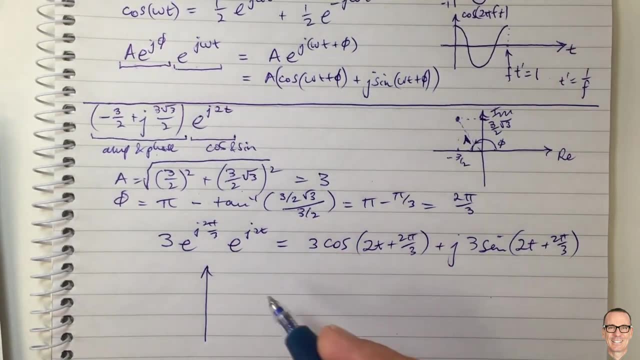 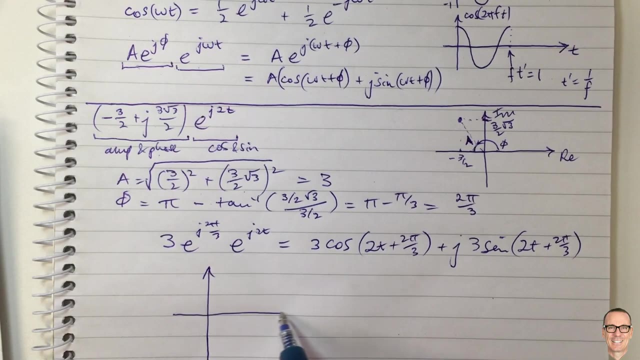 Okay, so this is going to be- let's do- the real part. So the real part is going to be a cos waveform that has an amplitude of three, So we can start plotting that here with an amplitude of three. Now let me fit this on here, on this curve, on this graph, here: 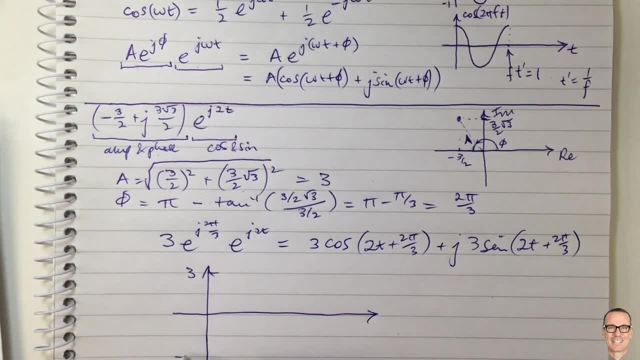 Okay, so it's going to have an amplitude. let's call that three and minus three. on my picture here It's a function of time, because it's cos. Now, what's the frequency? Well, here we can see the frequency out the front of the t. we've got a two. 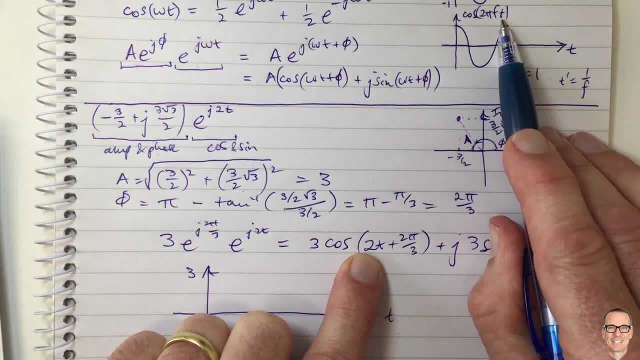 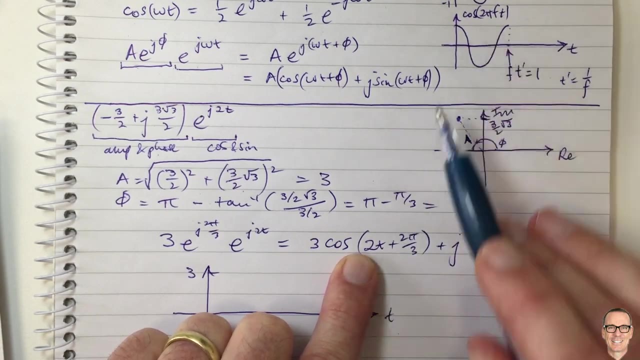 So up here we had two pi f out the front of the t, And so now we've got two So two. we can have this function here, where we're seeing that the two equates to the two pi f. So you can clearly see, here we can match up these two and we can then plot the same plot. 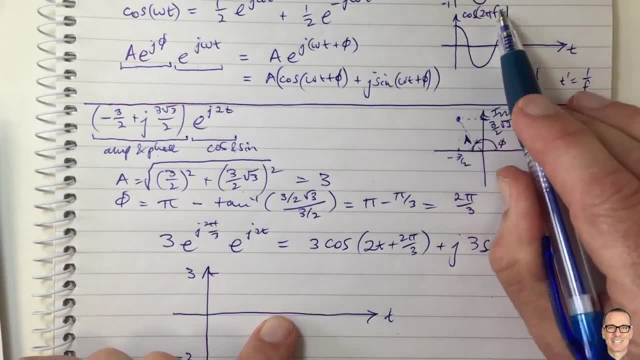 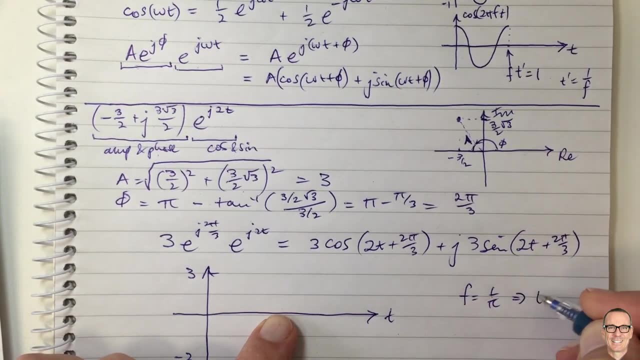 with that same frequency right there, when f equals one on pi. Okay, so f equals one divided by pi, which means the period equals pi seconds. So for this waveform here it's going to be two pi f, The period equals pi seconds. 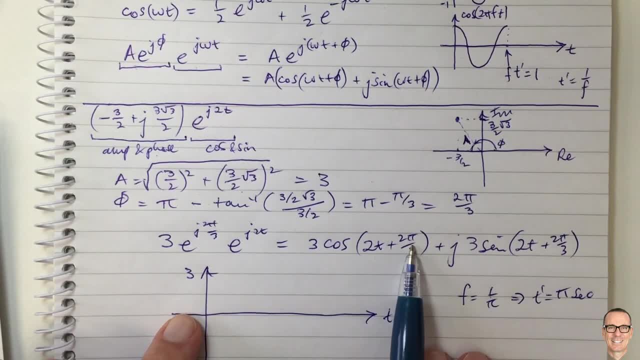 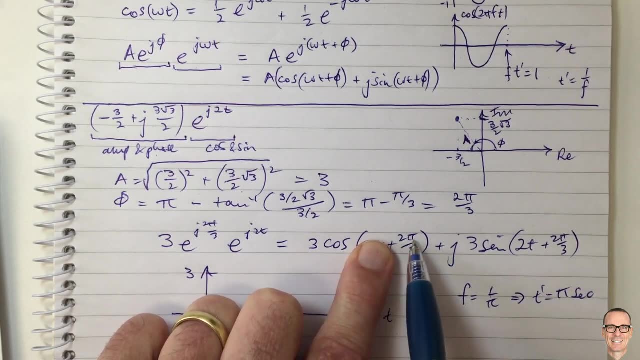 So that's the distance between the peaks, And then what's the phase offset? How do we work out the phase offset? Well, let's look. I always look when t equals zero. So when t equals zero, we've got cos of two pi on three. 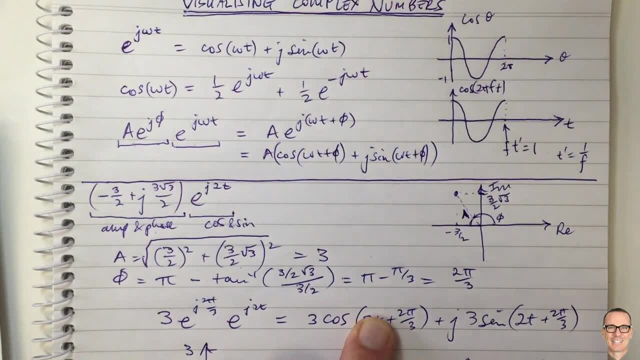 What's cos of two pi on three? Well, let's look back up to our thing here. There's cos of theta. So, when theta equals two, pi on three. when theta equals two, pi on three, well, where is that? Well, this is pi. 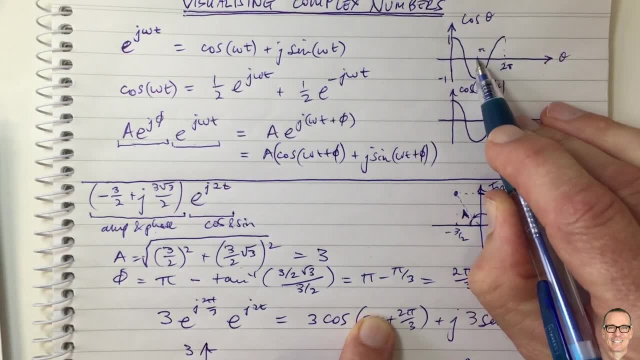 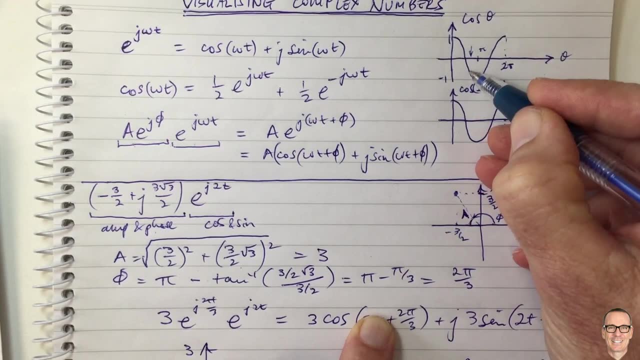 That was two pi. halfway along is pi. So now we've got two pi on three is two thirds of the way to pi. So that's in here, That there is two pi on three. So our waveform is going to start at that point there. 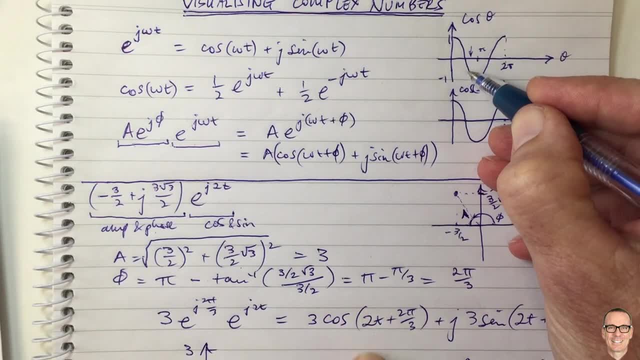 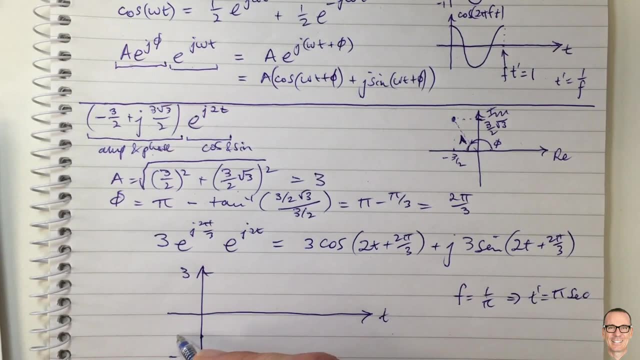 It's going to have a phase offset, which means it starts at that point there, When time equals zero. we have that point there, Okay. so that's this point here And you can work out. that actually is a half, So that's minus three on. two is the starting point. 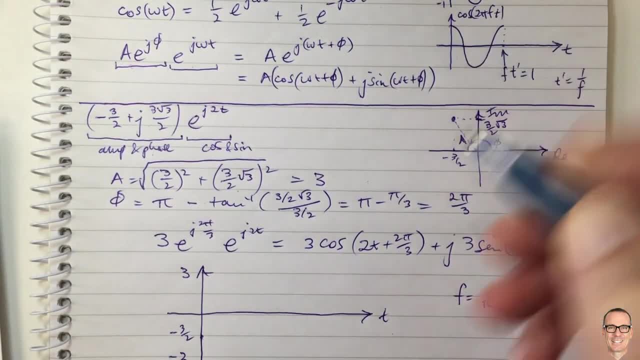 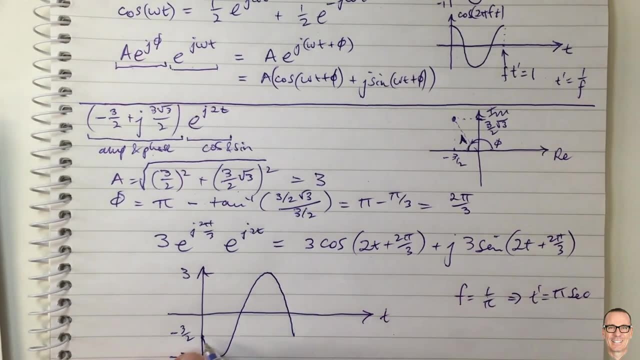 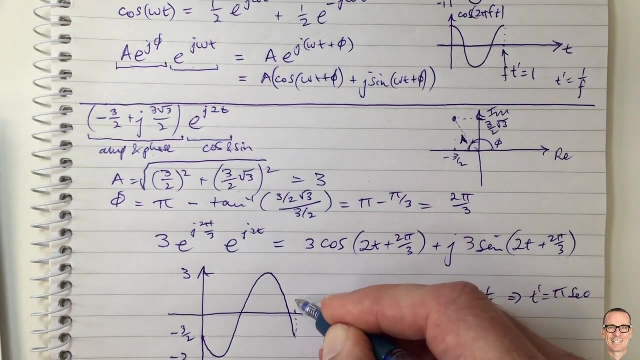 And then it's going to have this shape for the rest of the waveform. So it goes down to minus three, up to three, and back down here to minus three on two, And this then is one period, one full period. So that point there is a period and the period is pi seconds. 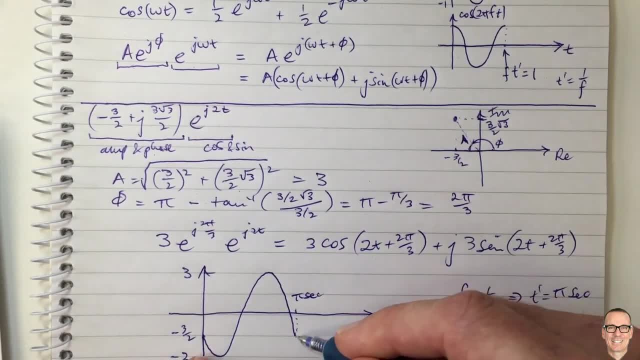 So that's pi seconds. So that is what this waveform is. Of course, it continues on, It's a continuing cos wave. And again, well, maybe I'll draw another version here to show you again: The period is pi seconds. 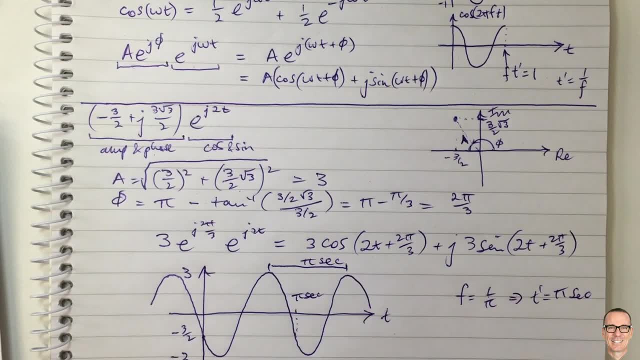 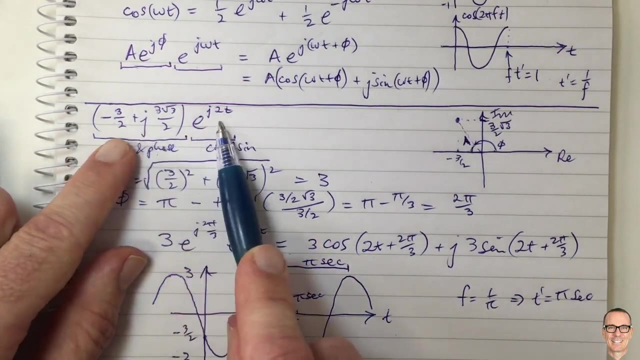 So that's pi seconds across between those peaks And this is the phase offset here that we've calculated because of this complex number that gave it a phase rotation. So hopefully this example has given you a bit of more insight into when you see the mathematics. 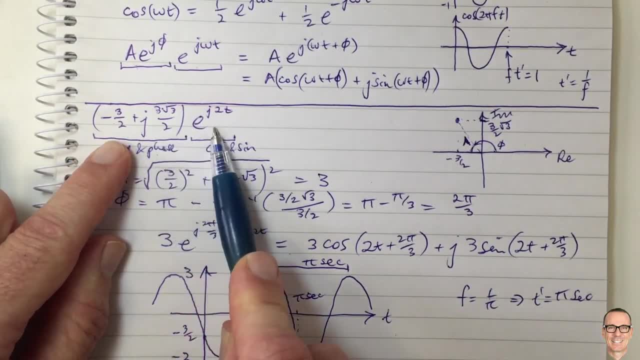 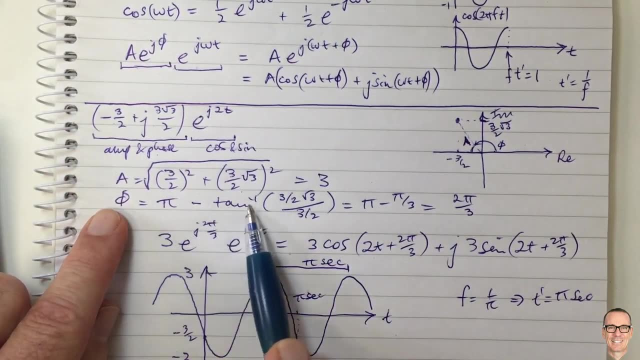 It's quite common for students to see this mathematics and simply start trying to apply the formulas that they're aware of. And if you did that, you may in fact find that you get into trouble when you do the arcturus Because you may not have realized about the phase being on the other side. 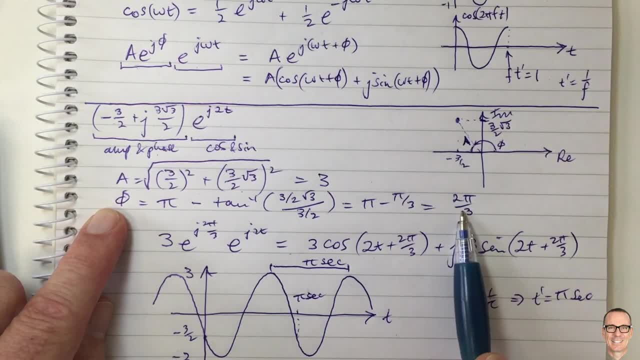 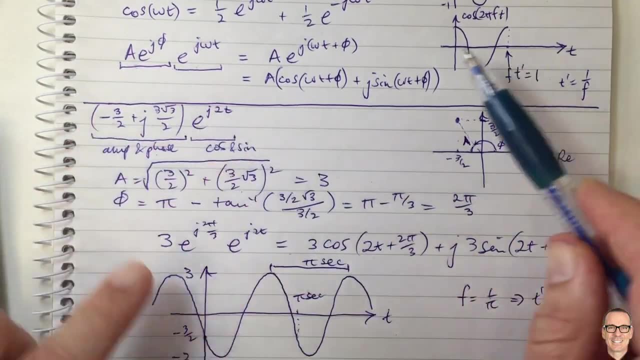 And you may end up with a pi on three instead of two pi on three, for example. So I always encourage you, whenever you see complex numbers, to think about what they are in terms of either a signal, if there's a time function like this up here. 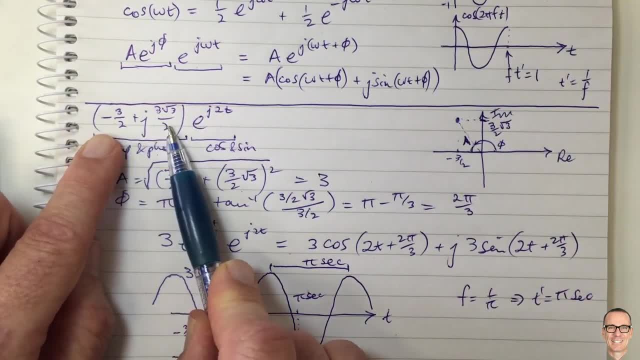 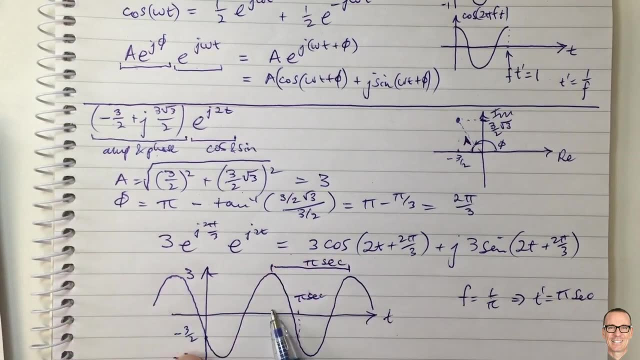 Or if they're an amplitude and phase, if they're something that doesn't have a time function, And think about what the final waveform is, or the final complex number in terms of waveforms of sines and cos. So if this has helped you to understand complex numbers, please give it a thumbs up. 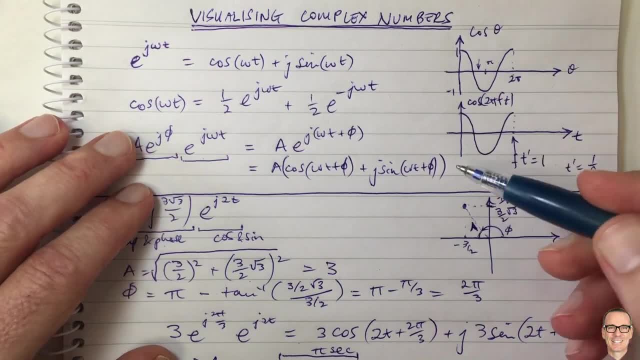 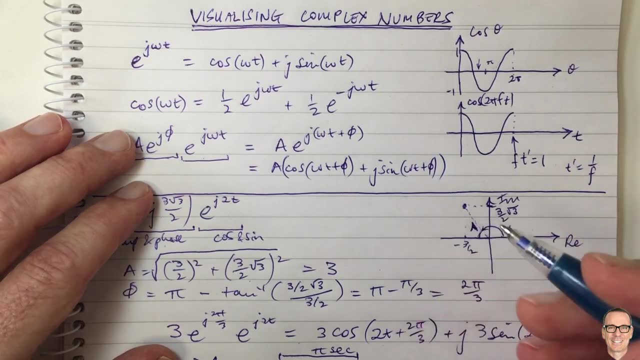 It helps others to find the video And subscribe to the channel for more videos And check out the web link in the information below the details below, where you'll find a full, categorized list of all the videos that are on the channel.